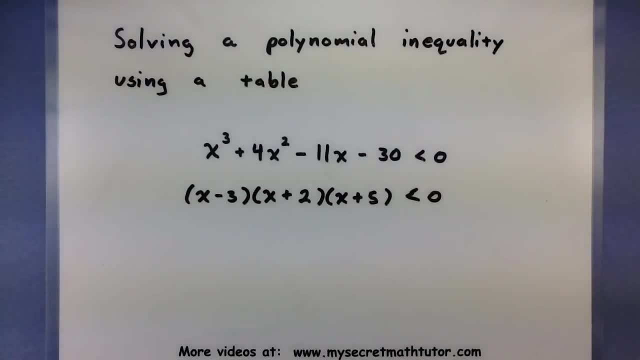 factors as a whole. You're going to have to do it in a different way. You're going to have to set them less than zero. That's not how you want to do this. Instead, let's figure out where each of these factors is equal to zero. Let's see. So the first factor would equal zero when x equals. 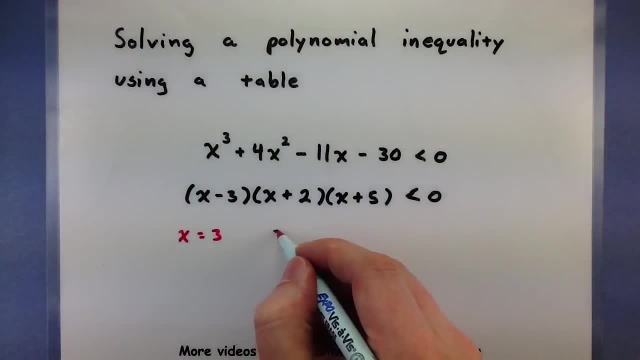 3.. The second one when x equals a negative. 2. And the last one when x equals a negative 5.. So you want to take each of these values and put them on a number line. We'll be checking around these values. We're going to take each of these values and put them on a number line. 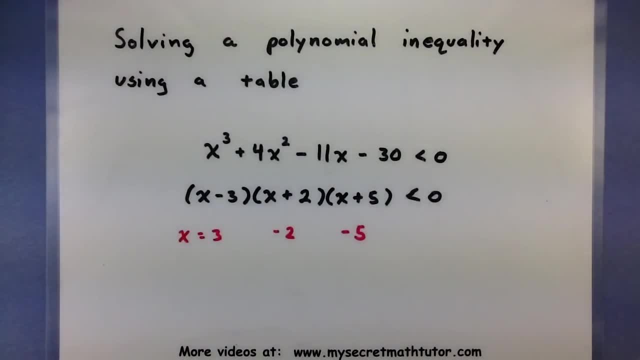 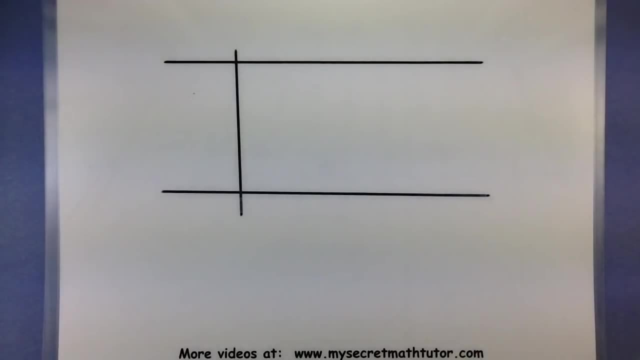 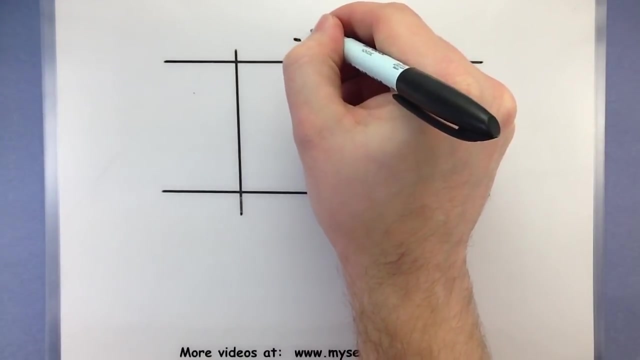 to figure out whether the entire thing is either positive or negative. All right, So I've already gone ahead and started to make this table already. Let's go ahead and put those values on there that we found. So I'm going to put them in the proper order. So minus 5 was: 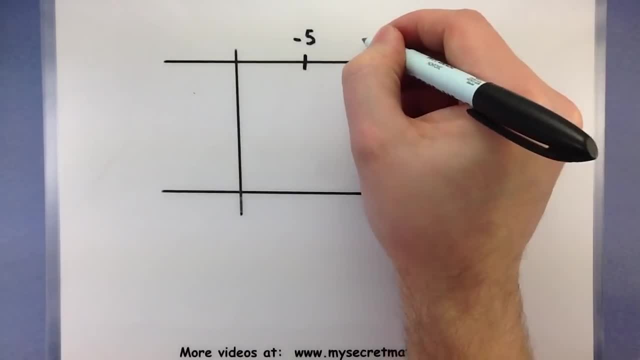 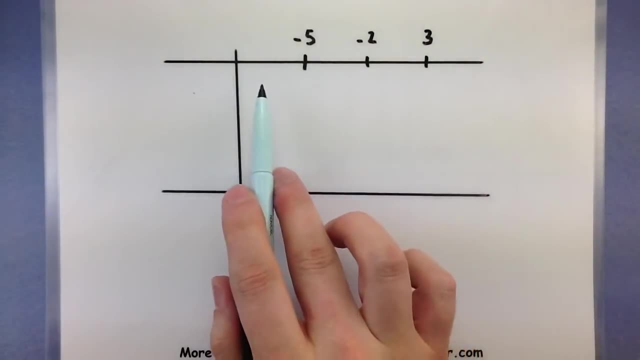 the smallest, followed by a minus 2.. And then there was a positive 3.. So this is like my number line. Now I want to see what's happening around it, So I'm going to take each of these values and count them, whether they're greater than 0 or less than 0.. Now, along this side of my table, go ahead. 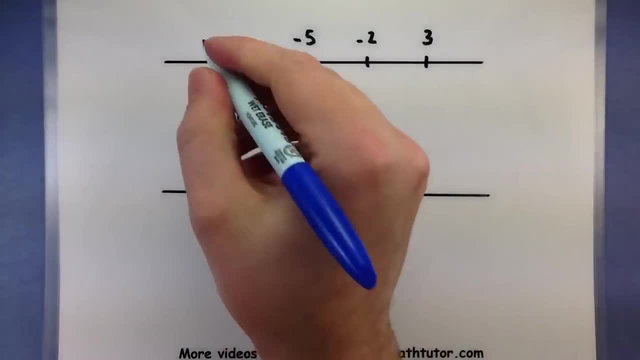 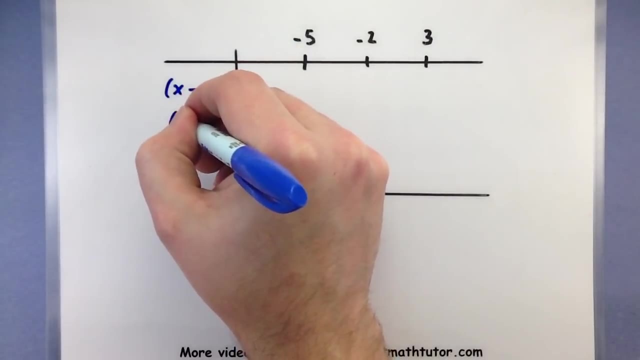 and put in the factors of your polynomial, So our factors, that when we broke this thing out, was x minus 3, x plus 2, and x plus 5.. This will just allow us to check the pieces of the polynomial, where it's positive, where it's negative, where it's negative. So if we were to select a number line, 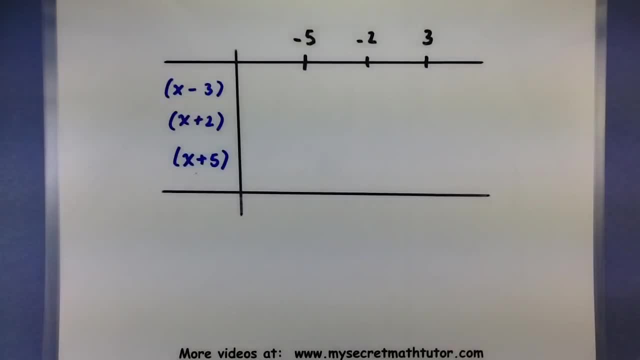 positive or negative, and I'll put it all together in the end. Alright, so now we want to take values around these zeros and test them in the appropriate factor. So let's pick something less than a negative 5, maybe something like a negative 6.. If I take negative 6 and I plug it into: 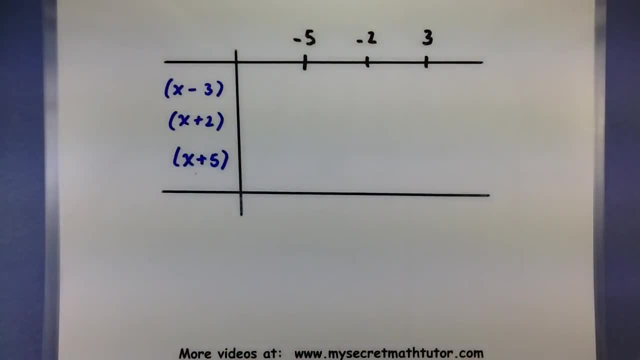 this factor, do I get a positive value or a negative value? Well, negative 6 minus 3, that's definitely negative. Okay, then I continue on to the next interval. so something between negative 5 and negative 2.. Maybe a negative 3 is a good one. What happens when I take a negative 3 and I put it into the 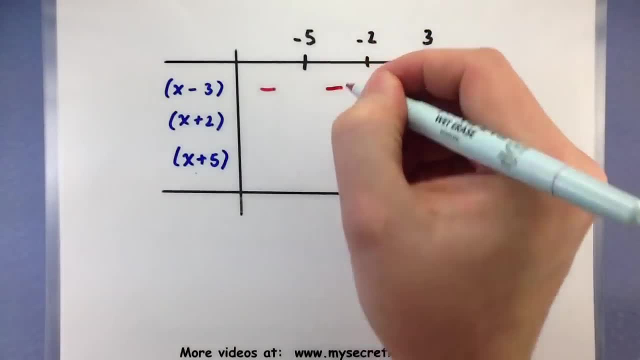 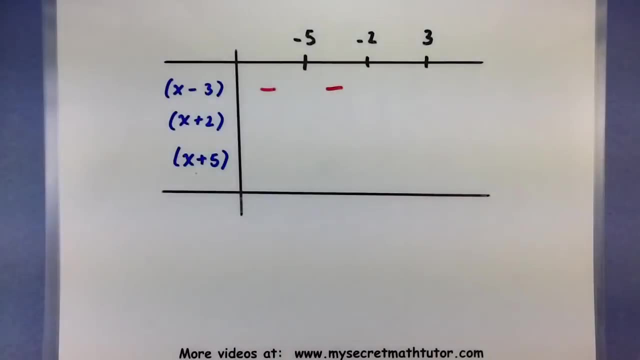 factor. Well, negative 3 minus 3, still negative. Pick something between negative 2 and 3, maybe 0 is good. Put it into the factor. so 0 minus 3 is negative And, of course, grab something larger than 3.. 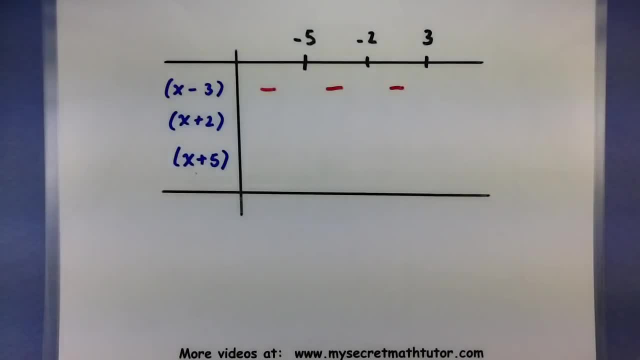 Plug it into the factor. see what you get. In this case, if I try something like 4, 4 minus 3 is positive. So this is keeping track of where this particular factor will be positive or negative. Now let's do that for the other two. 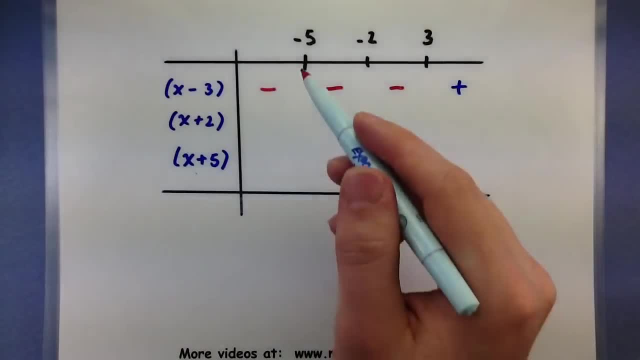 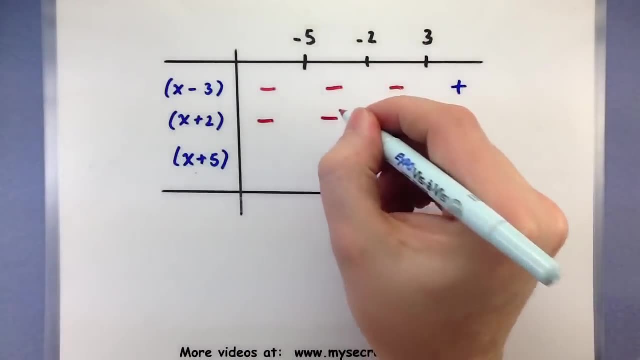 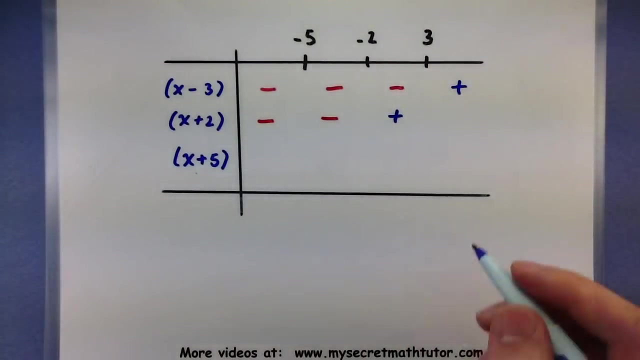 factors. So again, we'll choose something less than a negative 5,. we'll add 2 to it: still negative. Negative. 3 plus 2, still negative. 0 plus 2, is positive And something greater than 3 plus 2,. 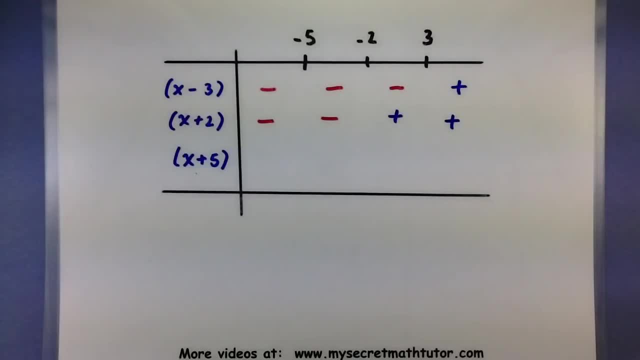 still positive. Alright, on to our last factor. Something less than a negative 5, plus 5, negative. Something between negative 2 and negative 5, maybe negative 3 will be positive. 0 plus 5 is positive: 4 plus 5. 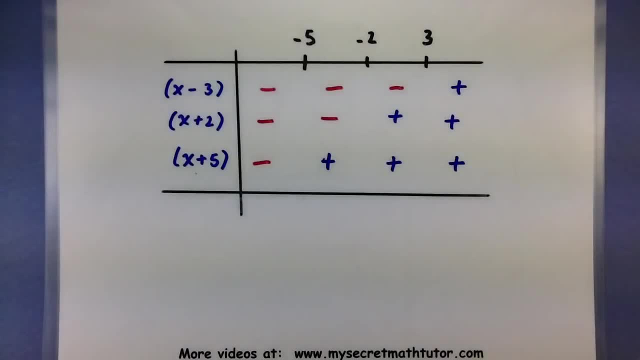 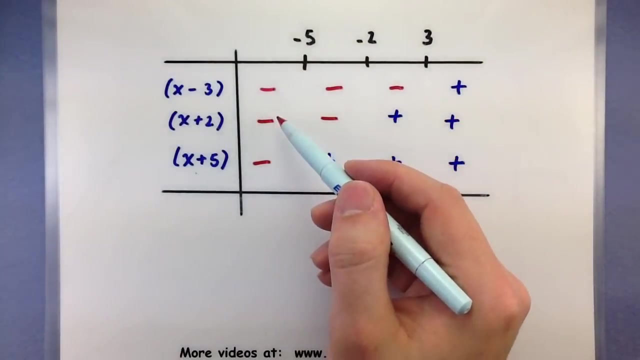 positive. So now I know what each of the factors will be around these zeros. Now, since each factor is being multiplied in the entire polynomial, I want to see what these will be multiplied together. So for the first interval I'll have a negative times. 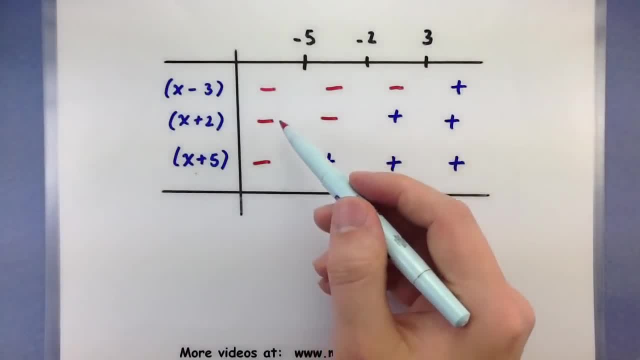 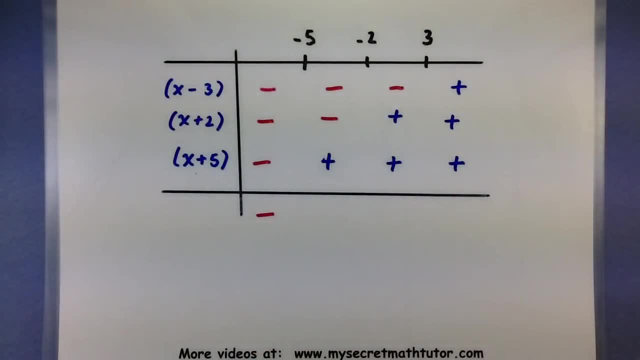 a negative times, another negative, Negative times- a negative would be positive Times, another negative, negative. This next interval, I have two negatives multiplied together, Then multiplied by a positive. So negative times negative. that would be positive times, positive, positive. 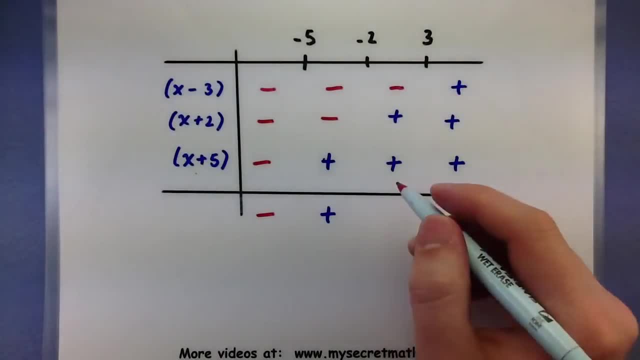 Now we have a negative times, a positive, so negative times, another positive, negative And, in my last one, positive times, positive times, positive. So this last row in the table corresponds to the entire polynomial And what we're looking for is: when is it less than zero? 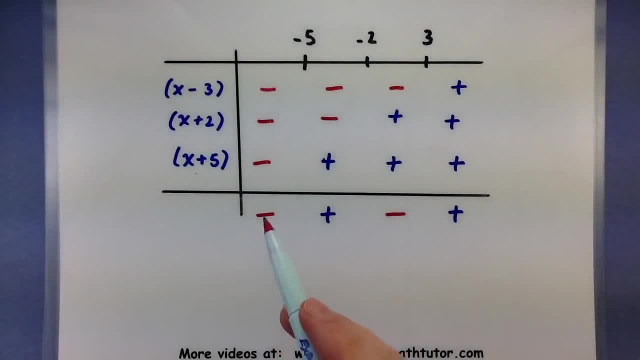 That's what our original problem was looking for, And so you can see this happens on two different intervals. Let's write down these intervals so we can represent our solution. So the first one goes from negative infinity all the way up to negative 5.. 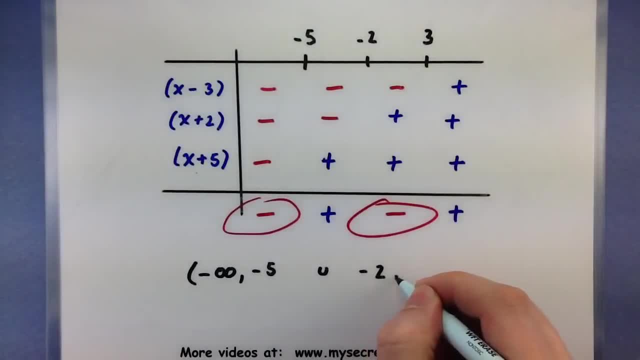 Then we go between negative 2 up to 3.. Now, since our inequality says when is it strictly less than zero? We don't want to include any of these endpoints, So I'll use the parentheses around these to show that they are not included. 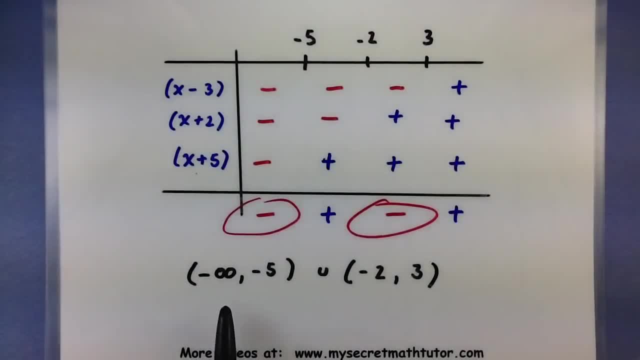 So the solution to my polynomial inequality is everything between negative infinity up to negative 5, and from negative 2 up to 3.. Now let's do one more example of this, just so you have the process down and you get better at using this table. 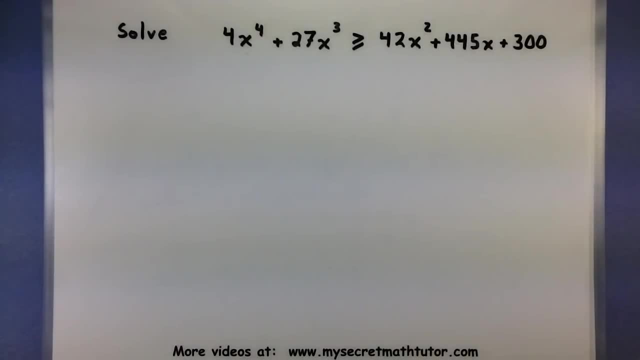 For this next example, We'll do a big one: 4x to the fourth plus 27x cubed is all greater than, or equal to, 42x squared plus 445x plus 300.. All right, With all of these inequalities, make sure you get them in relation to zero first. 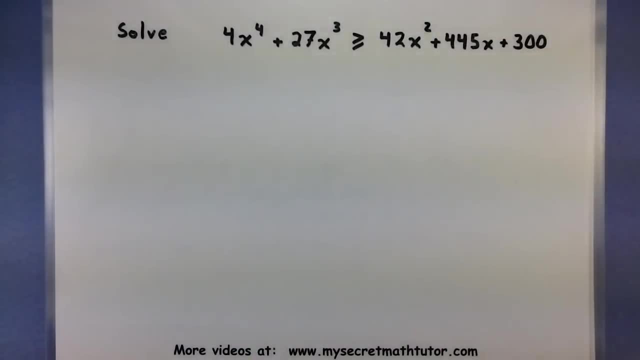 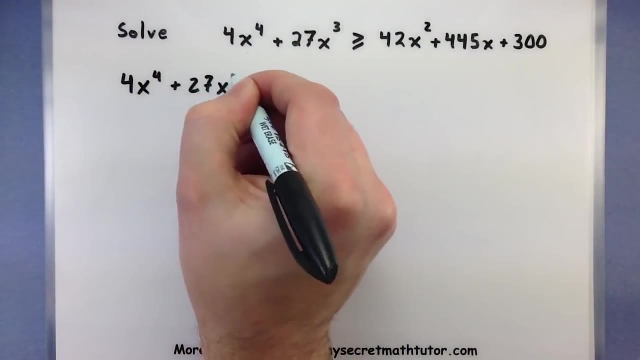 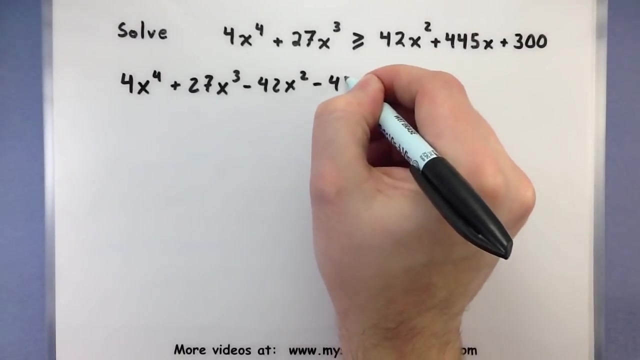 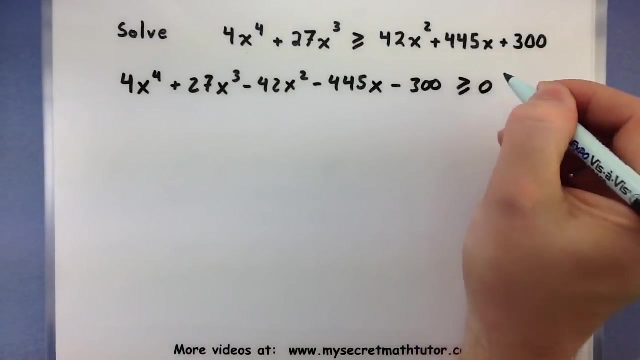 So I'm going to take all of these terms and subtract them over to the other side. That way I'll have a zero. So 4x to the fourth plus 27x cubed minus 42.. 4x squared minus 445x minus 300 is greater than or equal to zero. 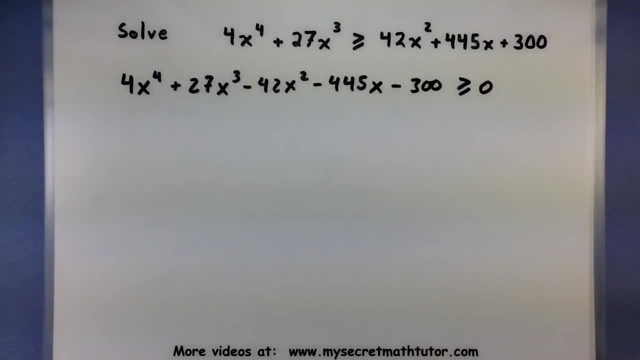 Awesome. Okay, Now here's where the factoring of polynomials comes into play. You would use your factoring techniques and break this into all of its factors. Now again, I've already done this before, So I'll go ahead and just list out the factors. 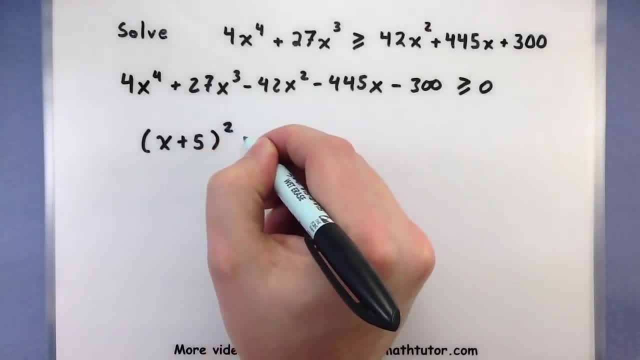 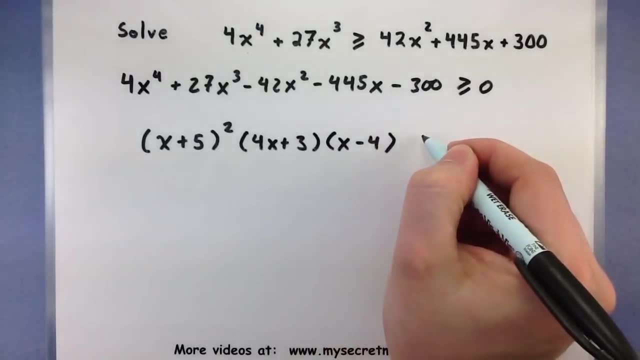 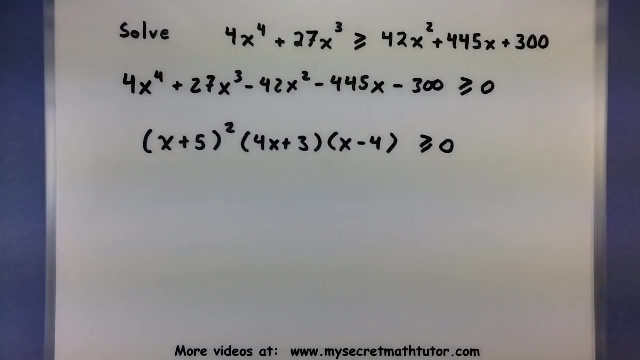 So x plus 5 squared 4x plus 3.. X minus 4, all greater than or equal to zero. So from each of these I want to figure out: well, where is it equal to zero? This one would be equal to zero when x equals a minus 5.. 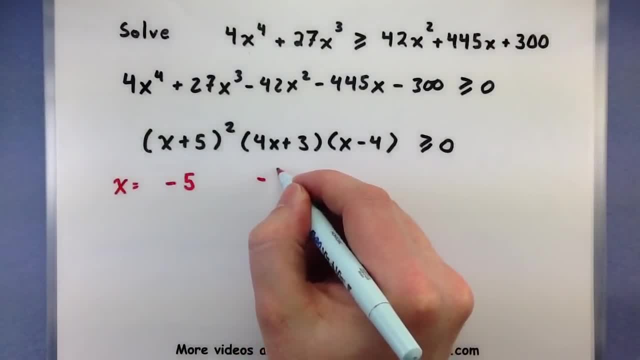 This one would be equal to zero when x equals a negative 3 quarters. Okay, All right. And the last one would be equal to zero when x equals 4.. So it's these points that I want to put on my number line, and it will also use these. 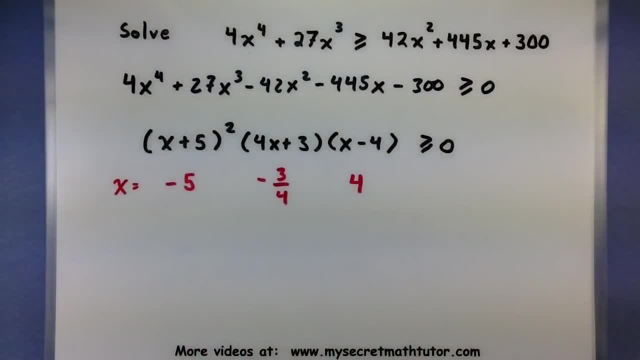 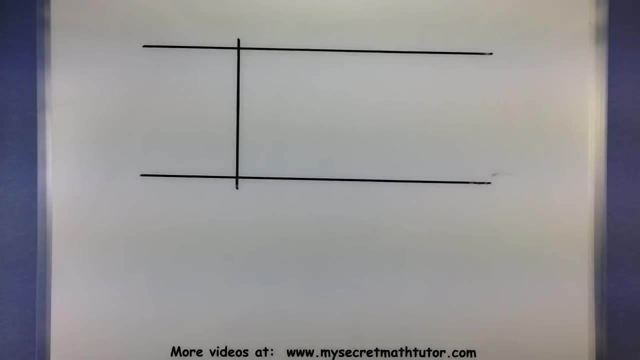 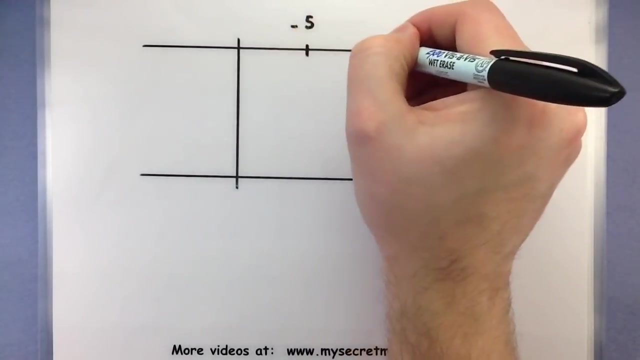 factors on the left side of our table. All right, Let's go ahead and put it all in. Remember to start off by writing the zeros on your number line, starting from the smallest all the way up to the largest. So our zeros were at minus 5.. 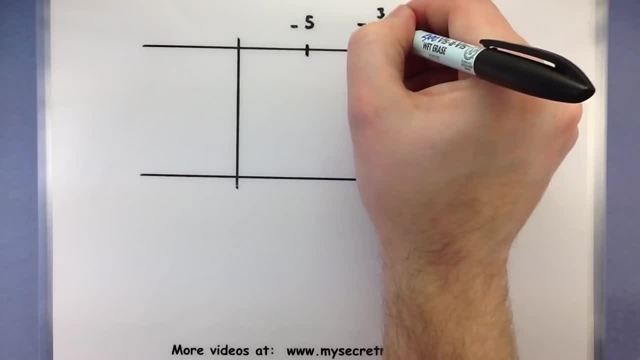 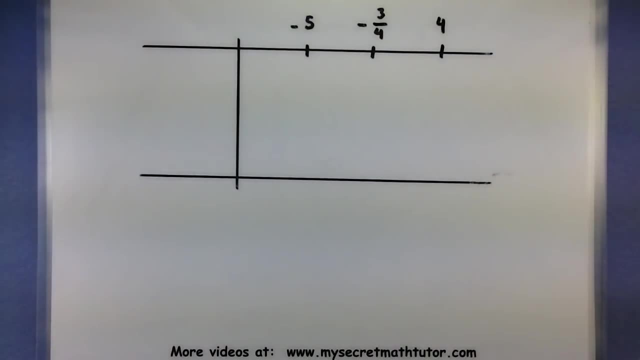 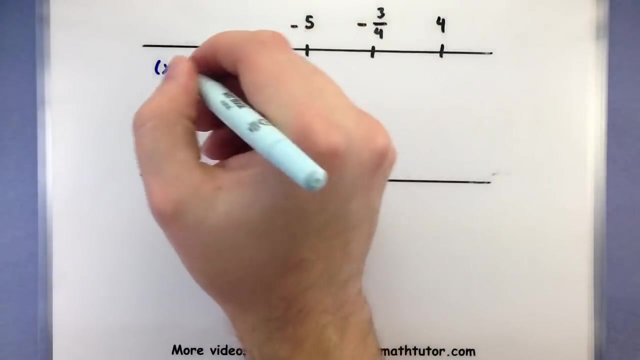 Minus 3, quarters and 4.. The factors that we'll be testing these in: x plus 5, squared, 4x plus 3, and x minus 4.. Awesome, Now here's where we're going to start. 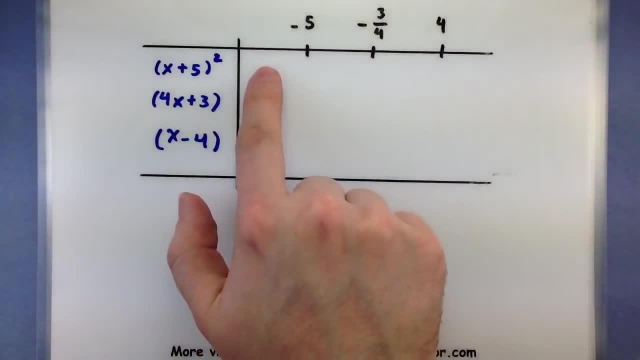 All right, All right, Let's start testing things out. We'll grab test points from each of these intervals, put them into the factor and we'll see if they are positive or negative. So let's pick something less than a negative 5, like maybe a negative 6.. 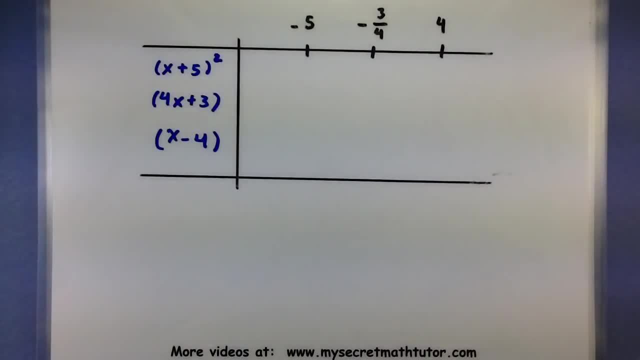 If I plug it in here, I'll have a negative 1 squared. Well, since it's being squared, it'll make it positive. In fact, you'll notice that, since this factor is being squared, no matter what I put in there, it will always make it positive. 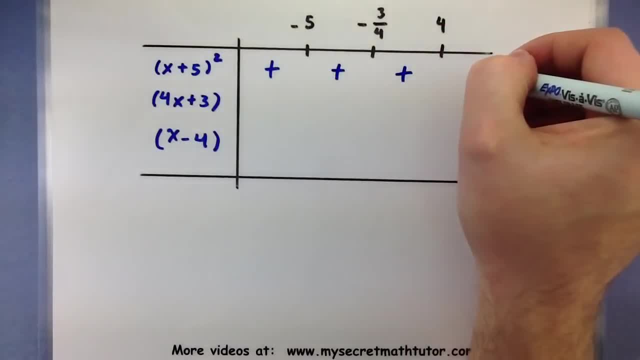 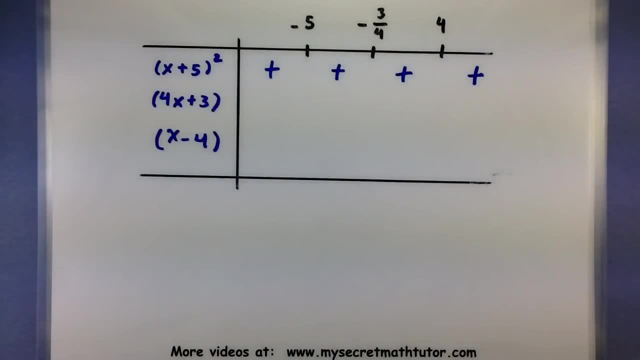 I'll make that one nice. All right, Let's try the next one. So what happens if I put a negative 6 into 4x plus 3?? Well, that will be negative. OK, Something between negative 3 quarters and negative 5.. 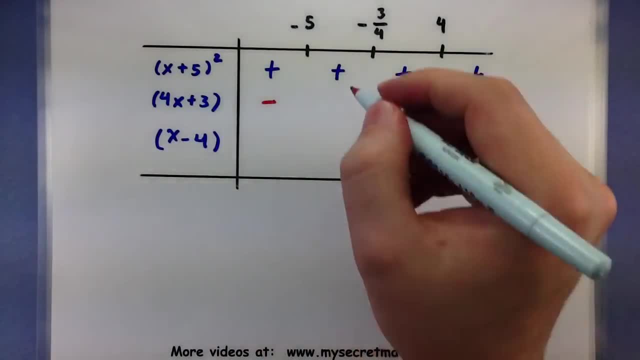 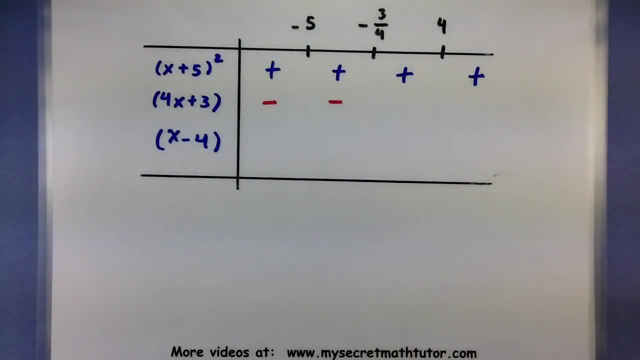 Maybe try a negative 1.. What happens when you put a negative 1 in there? Well, it's still negative. OK, between negative 3 quarters and 4.. Maybe 0 is a good choice. That would be positive, because 4 times 0 plus 3 is a positive 3. And something larger than 4, definitely positive Awesome. 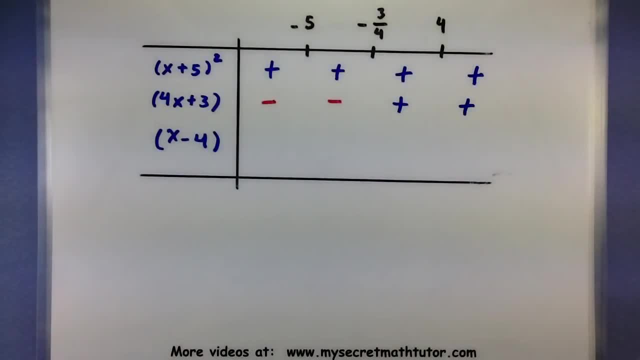 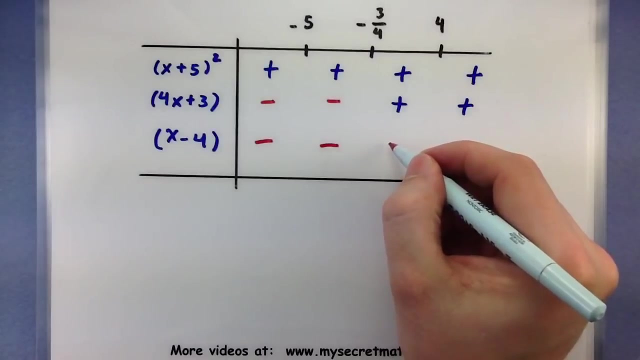 All right on to the last factor. Something less than a negative 5, minus 4, still negative, And something between negative 5 and negative 3 quarters. negative 1, minus 4, still negative. Between negative 3 quarters and 4, still negative And anything greater than 4,. 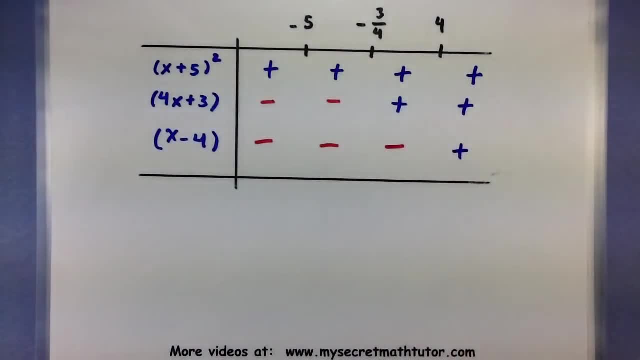 now it's finally positive. All right time to put all of this together. So all of the factors are being multiplied, so we will multiply all of our signs. So on the first one- positive times, negative times, a negative- Looks like we are positive. Positive times, a negative times, a negative: positive. 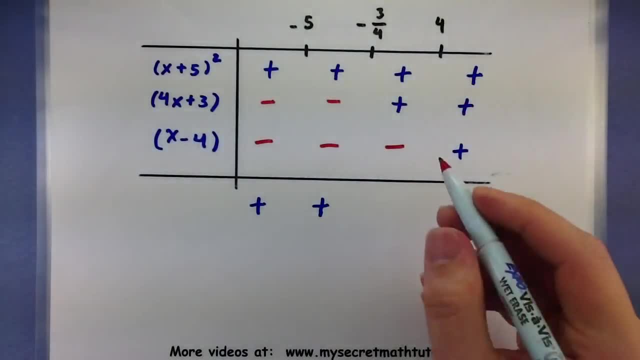 Now I have a positive times, a positive times, a negative, negative And the last one, a whole bunch of positive things multiplied together. positive, All right, looks good. Now, in this particular problem, we wanted to know where was it greater than or equal to 0.. 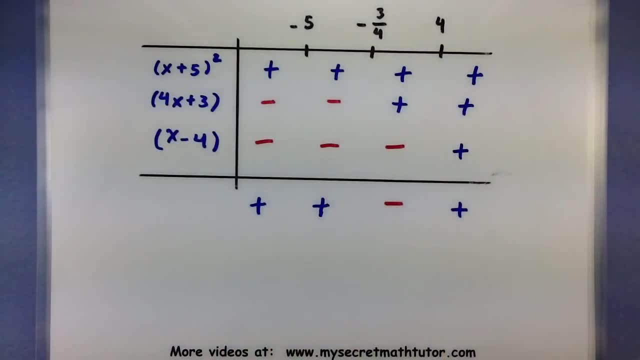 So let's first write down these intervals: where it was greater than 0,, definitely positive. So this one was from negative infinity up to negative 5, and from negative 5 up to negative 3 quarters, and then I had from 4 up to infinity. 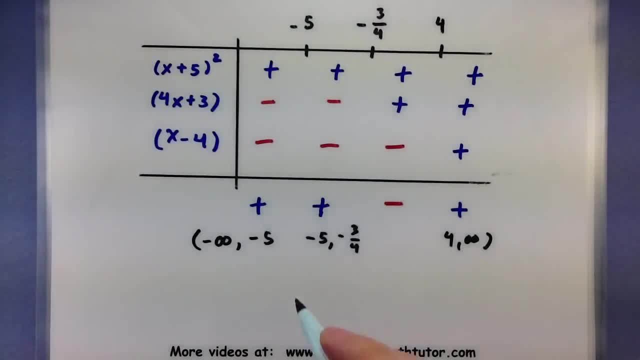 Now, since it said greater than or equal to 0, I would want to include each of these endpoints, Because at these endpoints it's actually equal. So I'm going to write down: this is equal to 0.. Put our little union symbols in here. 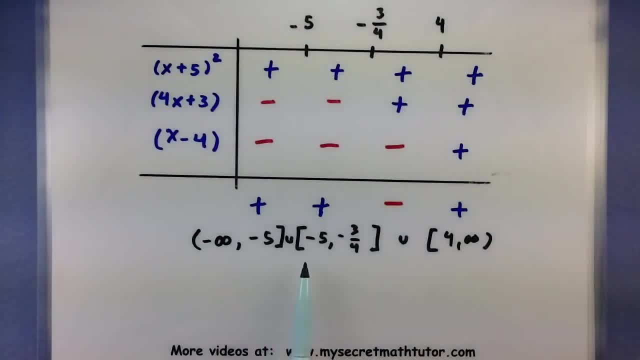 Now notice this one. the two intervals actually overlap. This one goes all the way up to negative 5.. It includes negative 5. And this one also includes negative 5 and then keeps going. So I'm just going to combine these two guys. 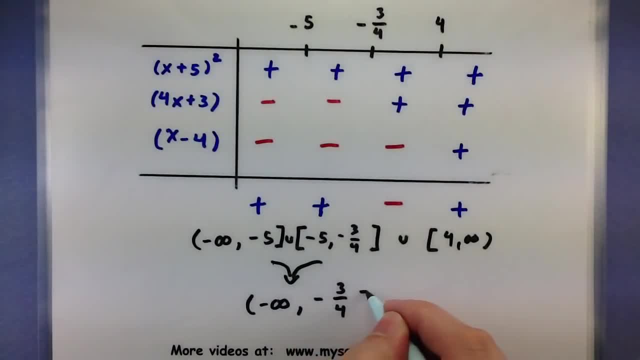 So negative infinity up to negative 3 quarters. So this entire section. they're all positive union for up to infinity. So this would be the solution to my polynomial inequality. If you'd like to see some more videos, please visit MySecretMathTutorcom.